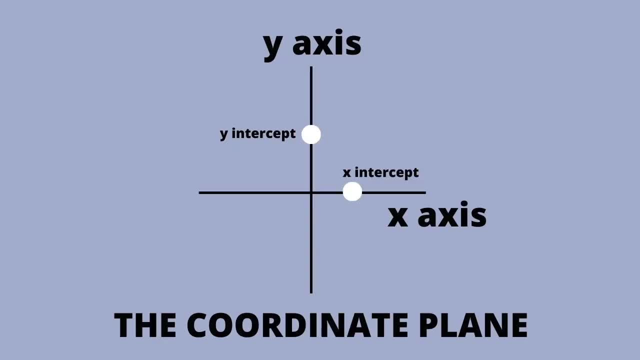 different letter combinations, but x and y are the most common. On the coordinate plane, the x-axis is where the independent variable is and the y-axis is where the dependent variable is. The x-intercept is where the function intersects the x-axis. The y-intercept is where the graph 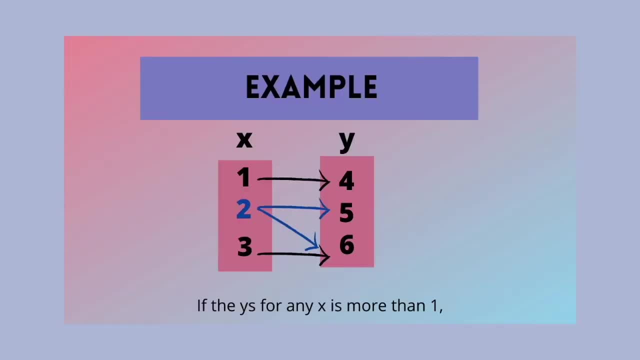 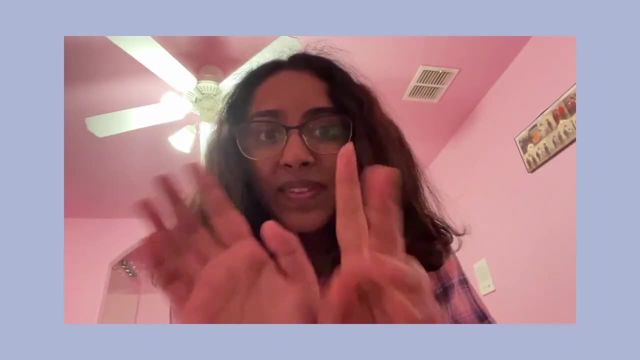 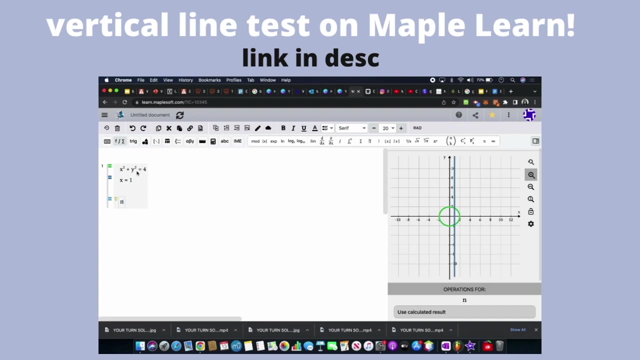 intersects the y-axis. But you have to keep in mind that if the y is 4 and x is more than 1, you do not have a function. There's an easy way to prove that a function is a function and it's called the vertical line test. You graph the function, you draw a vertical line If there's. 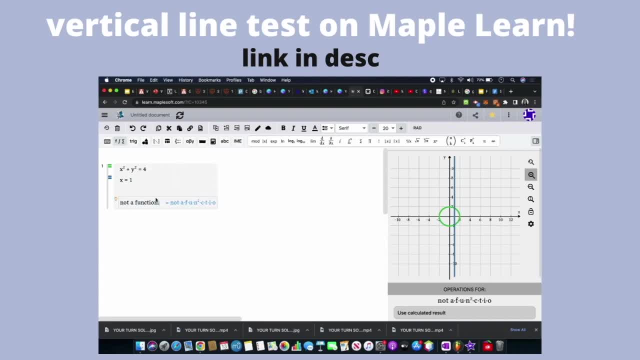 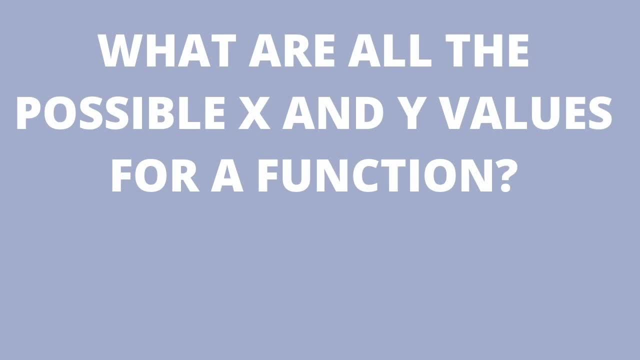 any two points that intersect with that vertical line. you know that you do not have a function. You can plug in random values of x to get their y values. but what is a way that we can determine all the possible x and y values for a function? It's called 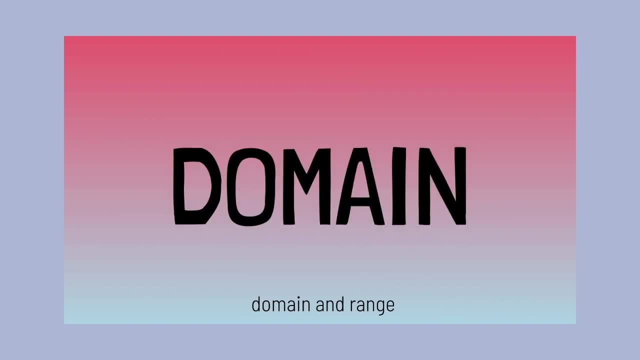 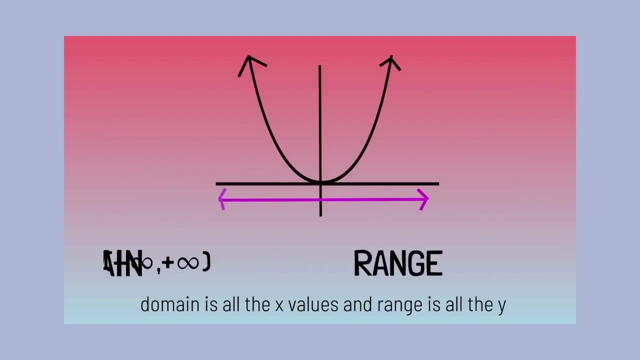 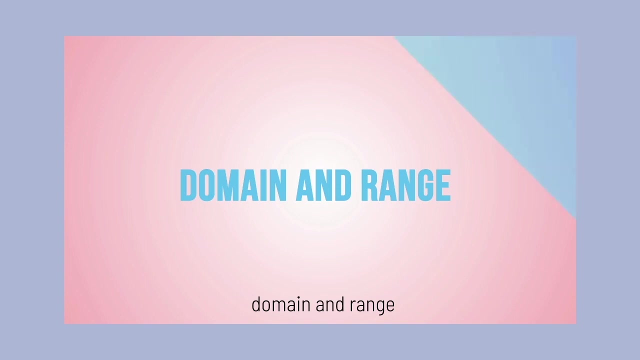 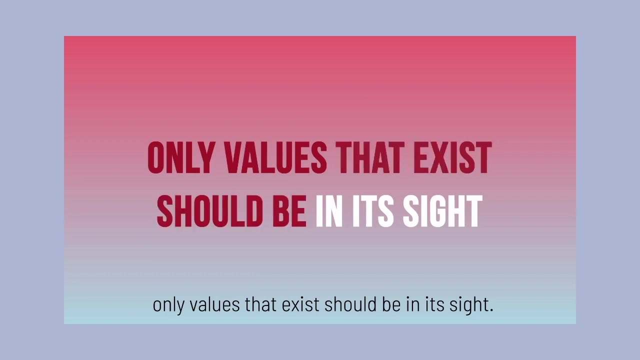 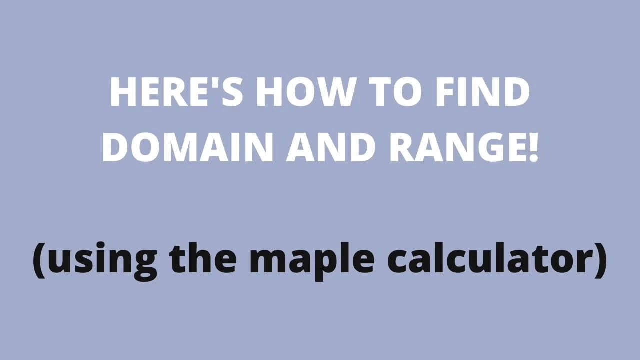 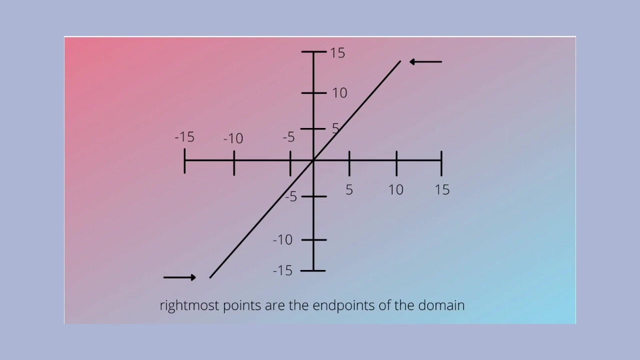 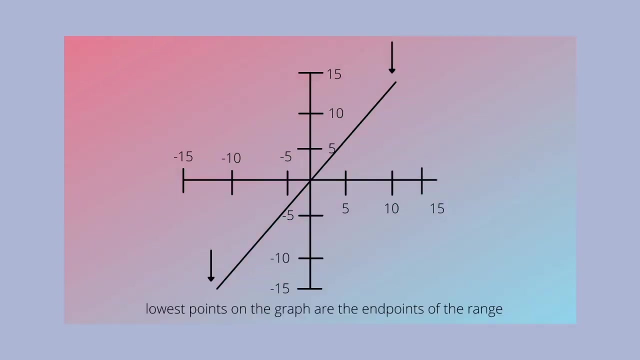 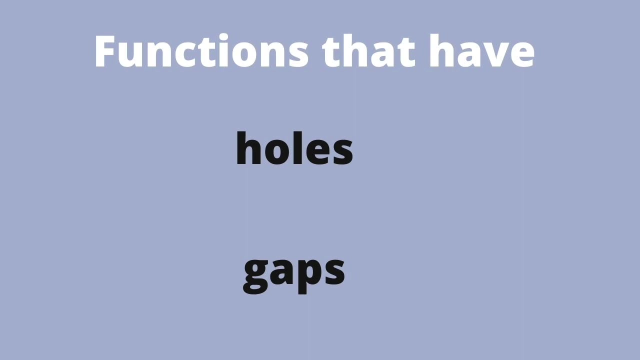 domain and range. If you have a function that's continuous, meaning that there's no holes or gaps, here's how to find the domain and range. det 천. Functions that may have holes or gaps in them instead are called piecewise functions, and how you would find the domain and range of those is. 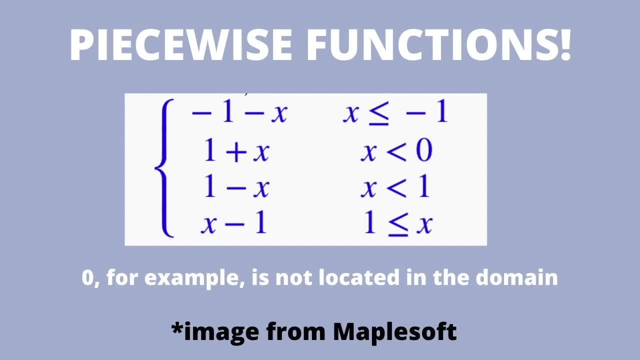 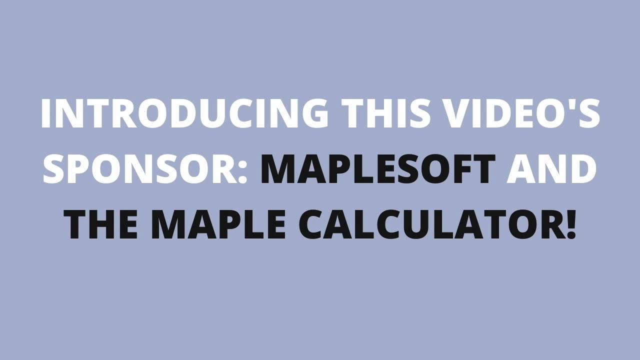 is. you could plot it on a graph or you could look at all the different pieces and find out where certain values and points are left out. we're now going to take a quick intermission and talk about our sponsor, maplesoft. if you feel absolutely unprepared for your algebra 1 eoc, keep listening. 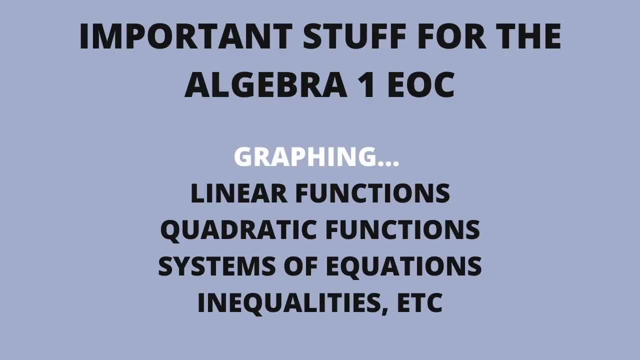 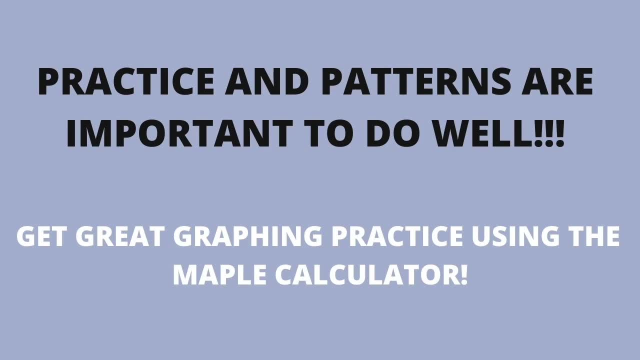 a huge part of the algebra 1 eoc is related to graphing linear functions, systems of equations, inequalities and everything that we just covered. practice and patterns are important to help you get a good score. get easy graphing practice using the maple calculator: open the app and click on the. 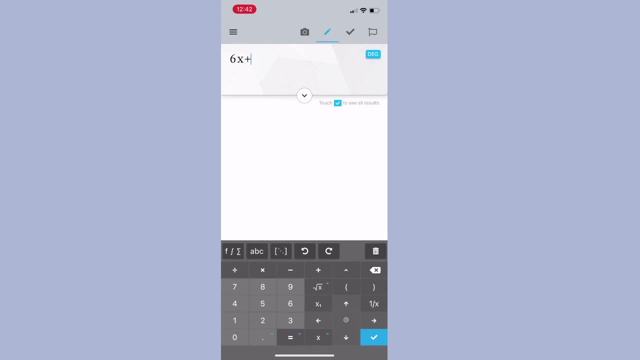 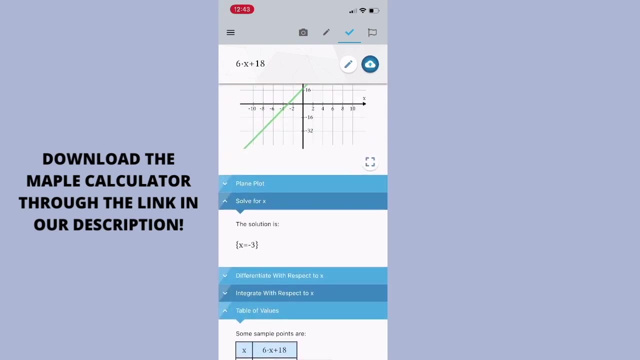 pencil icon, plot any equation and a graph will appear below it plotting the equation. next, visit the check mark icon to see how to plot the equation, how to solve for x, and you get a table, and some even allow you to see a 3d model of your graph, which is pretty fun. have fun graphing by. 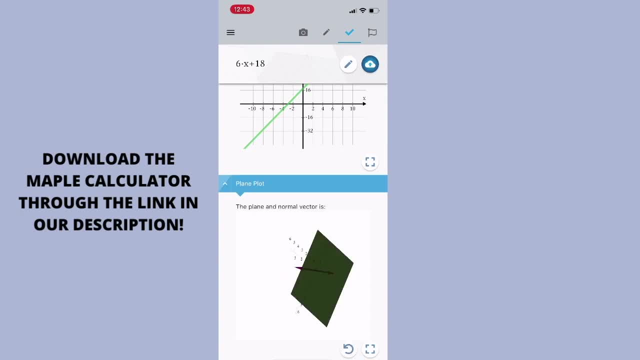 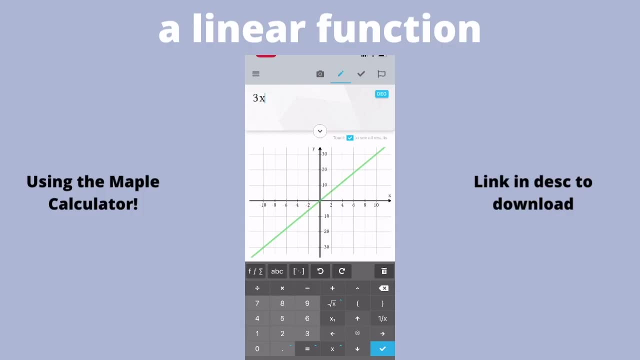 downloading both the calculator and maple learn in our description below. let's now get into the main functions that you should know to succeed in algebra 1.. the first one is called a linear function. it's a straight line. i'm gonna be fine. i'm pretty sure y'all are familiar with the phrase. 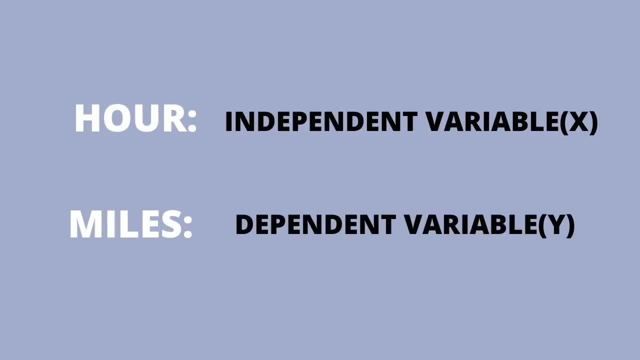 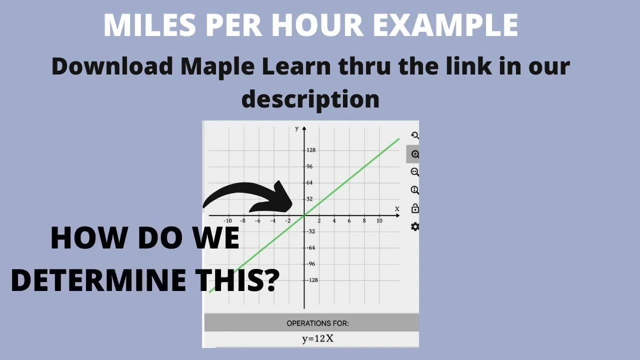 miles per hour. uh, hour is the number of miles per hour and hour is the number of hours per hour, the independent variable, and miles is the dependent variable, and the relationship between these two can be represented as how steep a linear function is. how do we determine the steepness of? 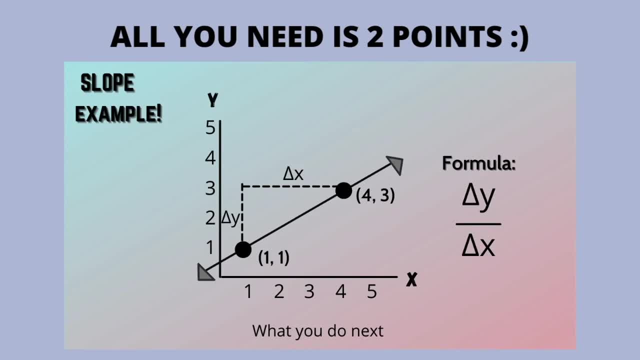 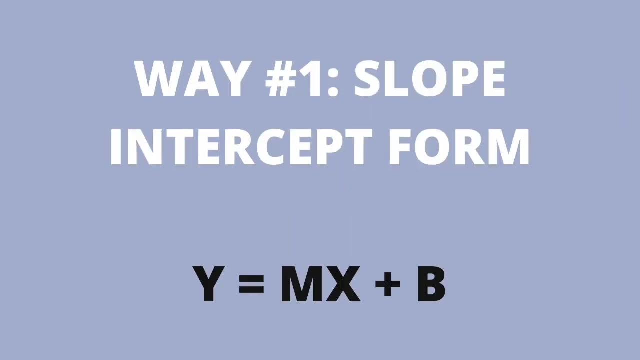 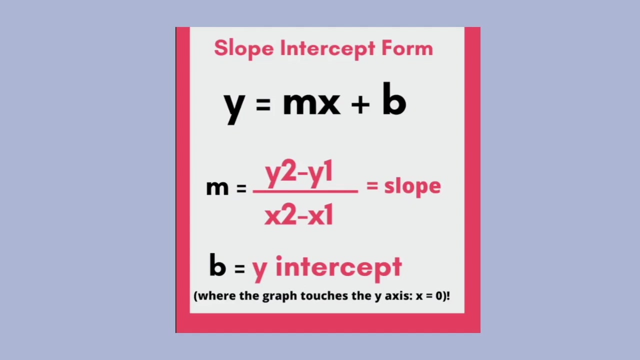 a graph. it's called slope and what you do next is take the change in y divide by changing x. another name for slope is: linear equations always have a constant slope and there are three different ways that you could write a linear equation. exhibit a slope. intercept form: y is mx plus b, y is mx plus b and there's a slope of the line. 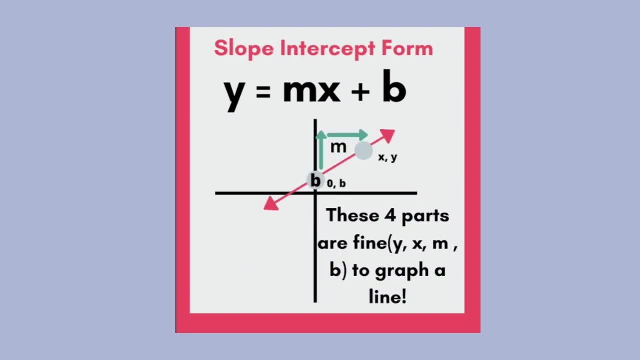 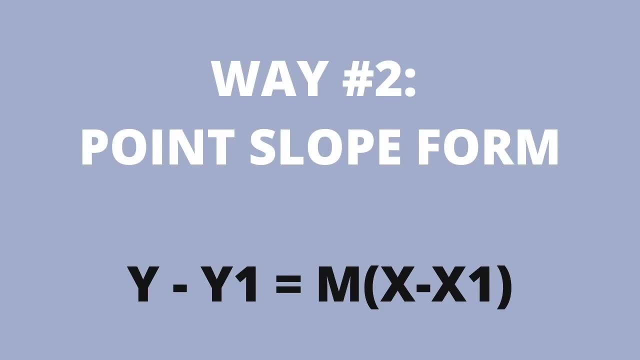 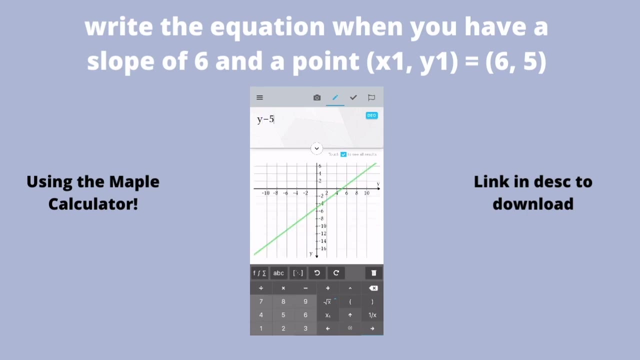 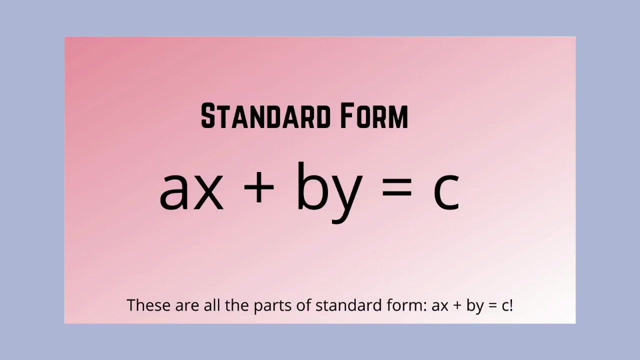 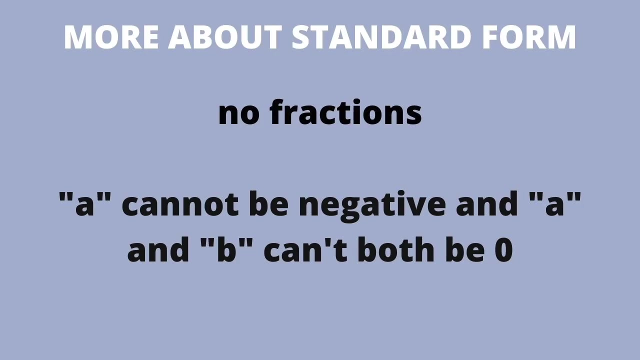 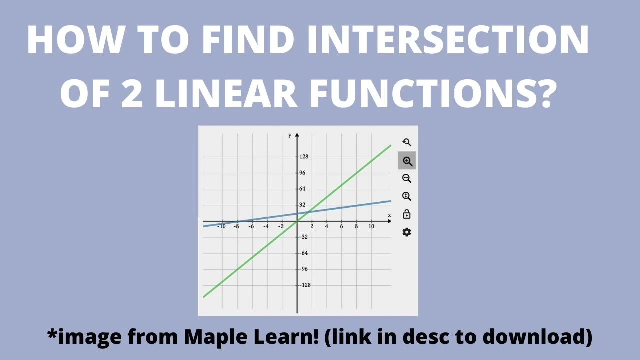 while b is the y intercept, y is mx plus b, y is mx plus b. these four parts are fine to graph. a line exhibit b: point slope form eat: is is the slope. So that wraps up three forms of linear equations. Now what do we want to do if we want to find out where two linear functions intersect? 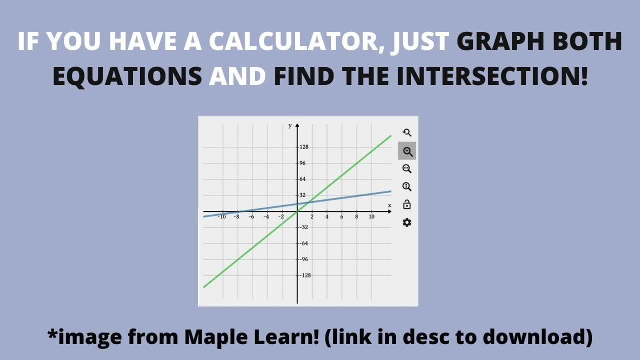 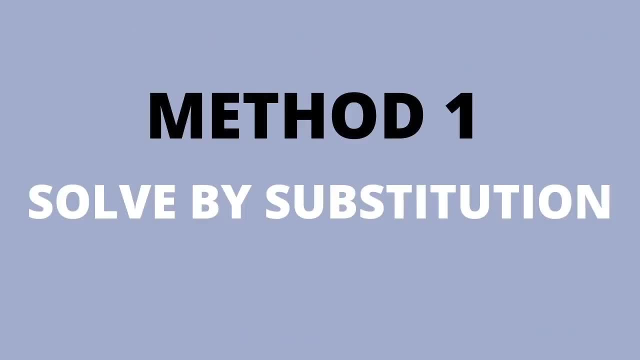 We now have a system of equations. If you have a calculator, just graph both equations and see where they intersect. Simple, easy, but it's good to know the other ways to do it as well. Method one is substitution. To solve an equation using substitution, you would write one variable in terms of the other. 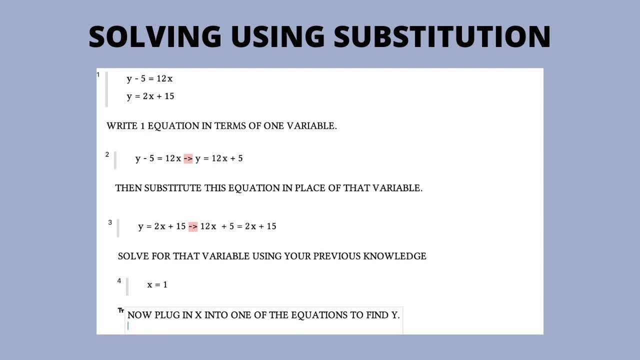 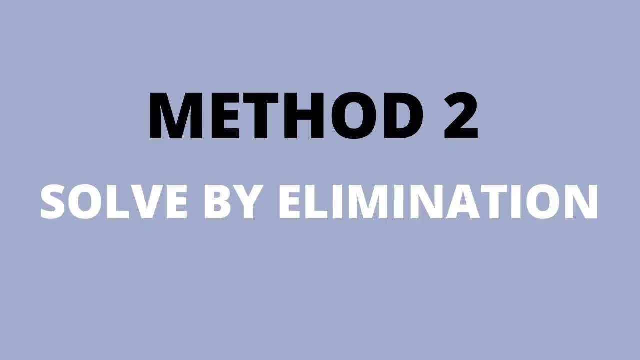 So if you have y equals x plus 5, wherever you see y, you just replace it with x plus 5, solve for x and then plug that x back in and then solve for y. Method two is elimination. To solve using elimination, you just eliminate one of the variables. 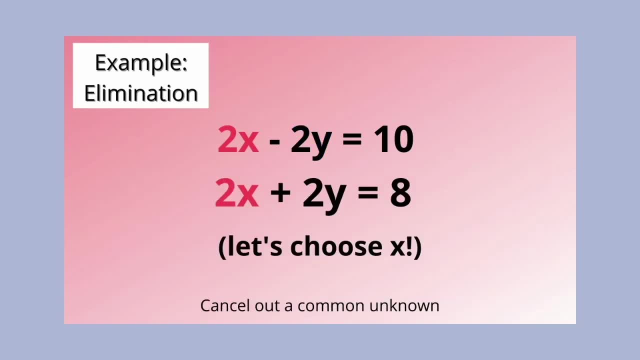 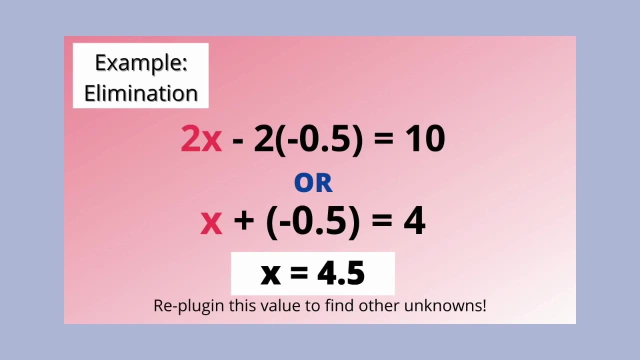 So you line up both equations so that both coefficients and letters match, and then you have to try to figure out some way to cancel out one of them. solve for one of the letters and plug it back in to solve for the other one. 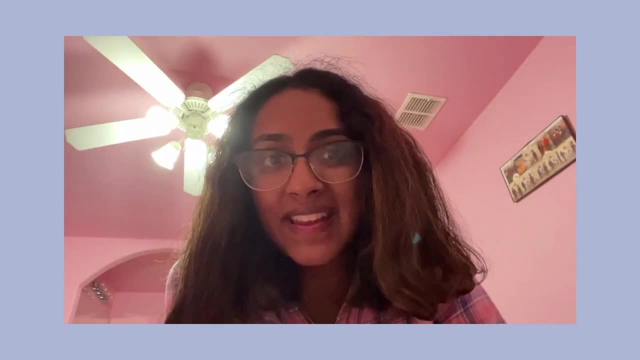 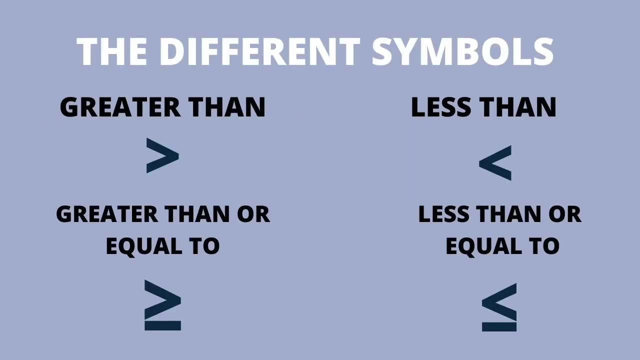 Before we wrap up linear functions, let's talk about linear inequalities. I mentioned that linear equations have to be equal to each other on both sides, but that's not necessarily true. with an inequality, You have greater than, less than, greater than or equal to, or less than or equal to. 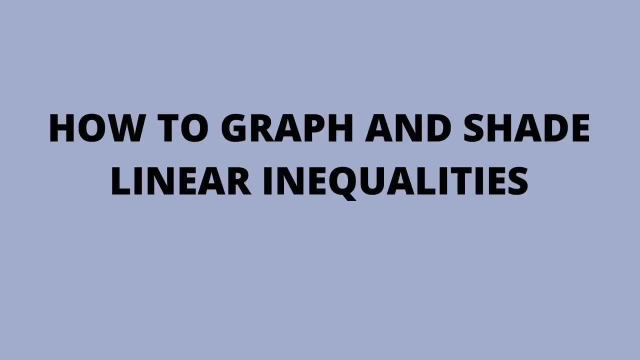 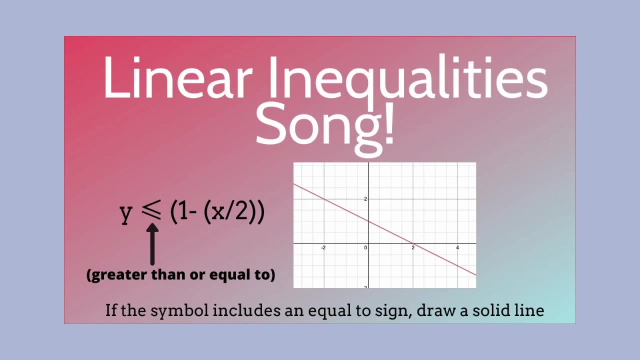 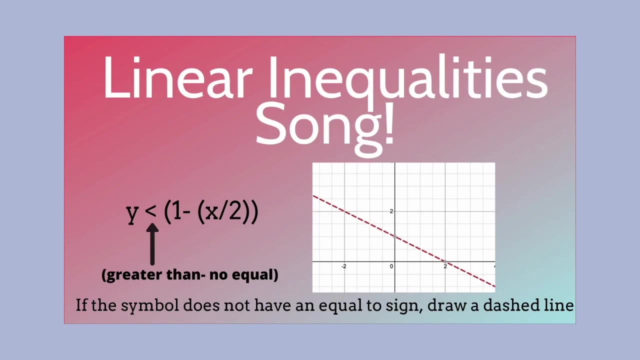 and you basically follow what the sign says. And here is how to graph and shade linear inequalities on a graph. If the symbol includes an equal to sign, draw a solid line. If the symbol does not have an equal to sign, draw a dash line. 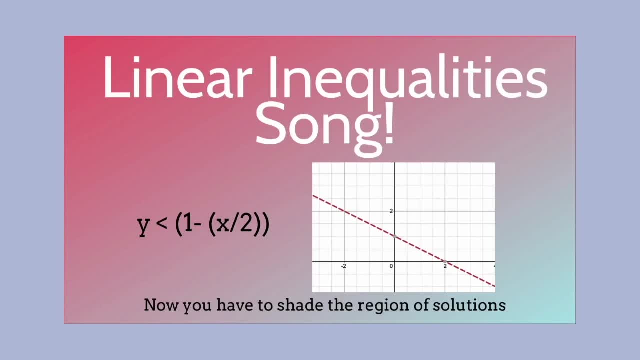 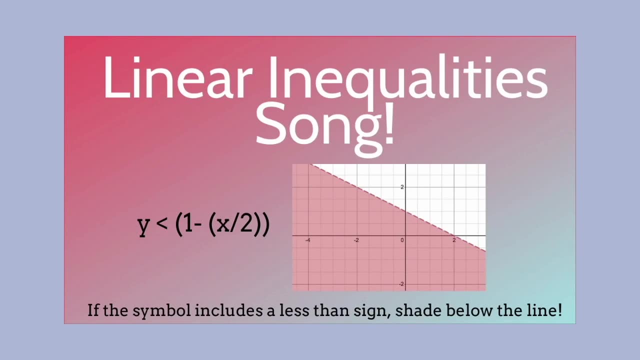 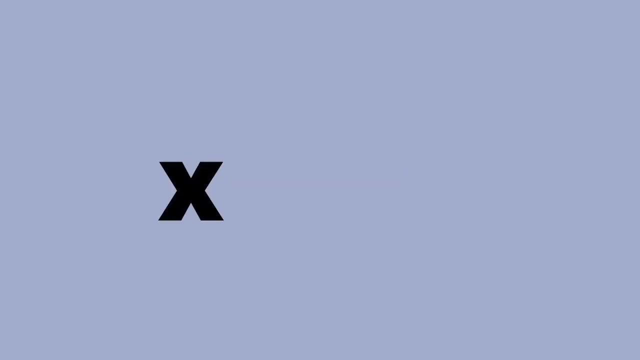 Now you have to shade. Oh, Here is the second main function that you have to know. We have linear functions. but what happens if we take x and we multiply it by itself? It becomes x squared, and this is the basis of a quadratic function. 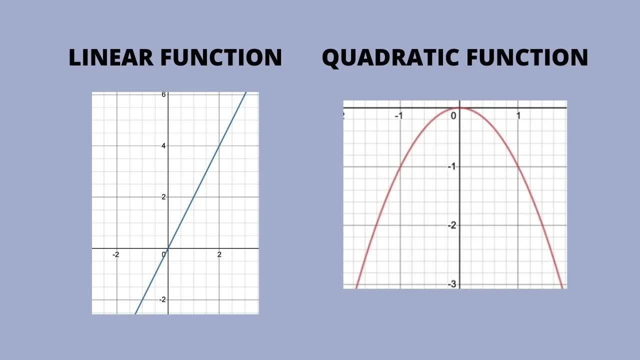 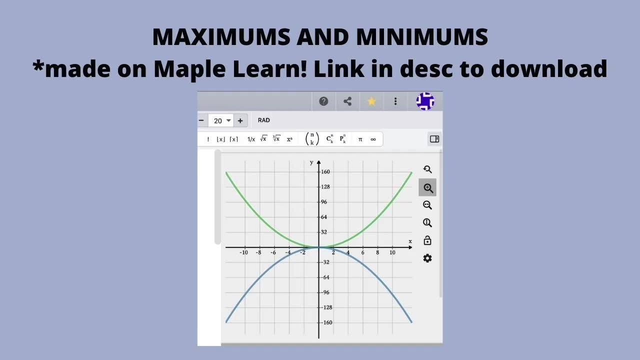 And, unlike linear functions, these aren't lines. All of these are u-shaped and they have an infinite domain, just like linear functions, but the range is limited because a u-shape has either a maximum point or a minimum point, depending on whether it's facing upward or downward. 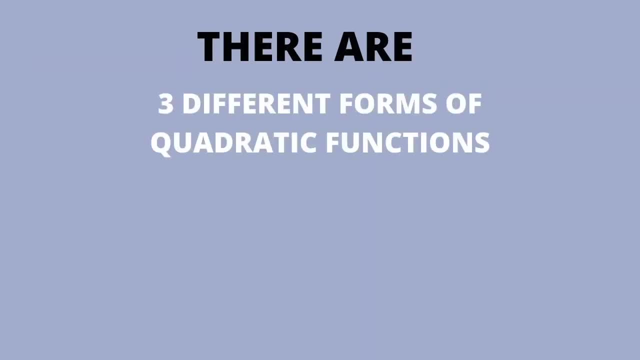 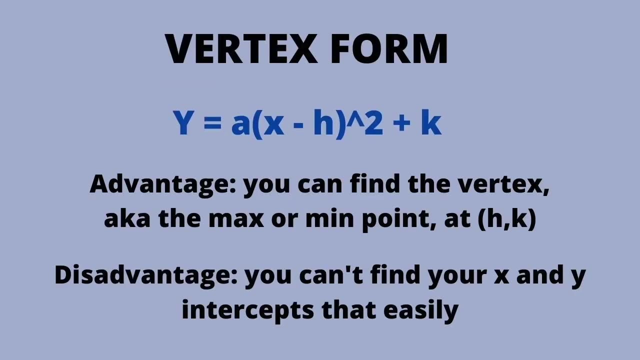 There are three different forms of quadratic functions: vertex, standard and factored form. Each form has their own advantages and disadvantages. The vertex form helps you find the vertex, which is h comma k. For standard form, 0c is the y-intercept. 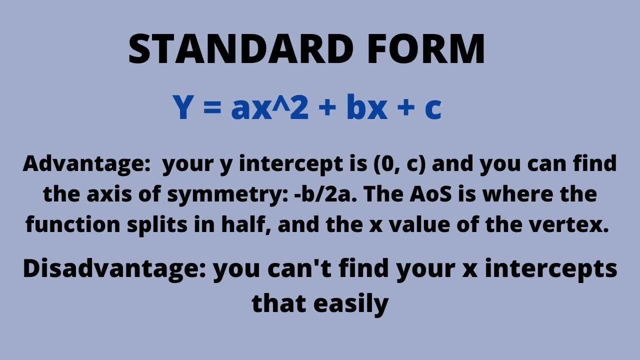 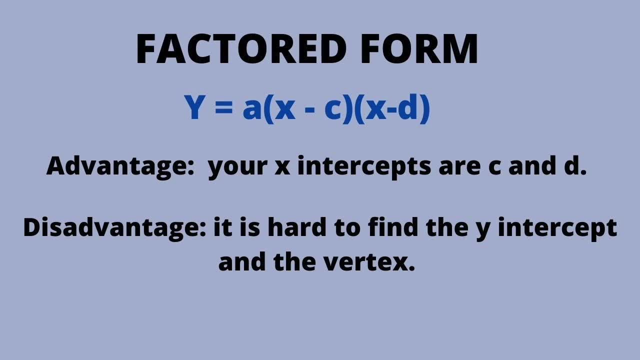 and negative b over 2a is the x-value of the axis of symmetry, which is where the graph splits in half. Factored form helps you find your zeros, your roots, and it's also called your x-intercepts. So how do you solve for the zeros? 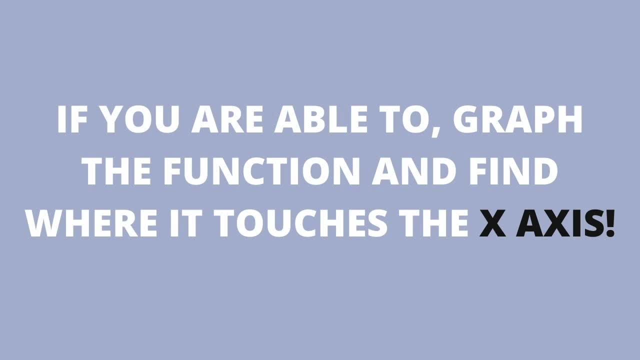 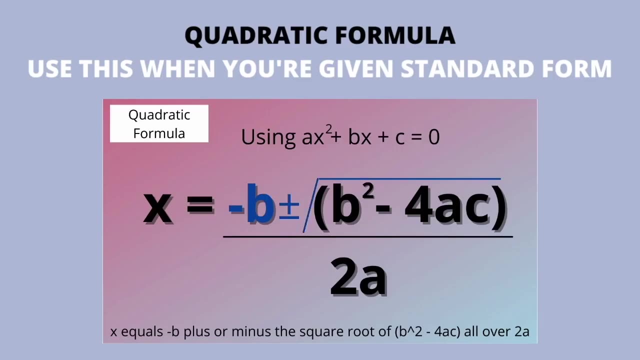 The first step is: you could obviously graph it if you have a calculator, and see where it intersects the x-axis. And obviously we cannot forget x is equal to negative b plus or minus, the square root of b squared minus 4ac, all over 2a. 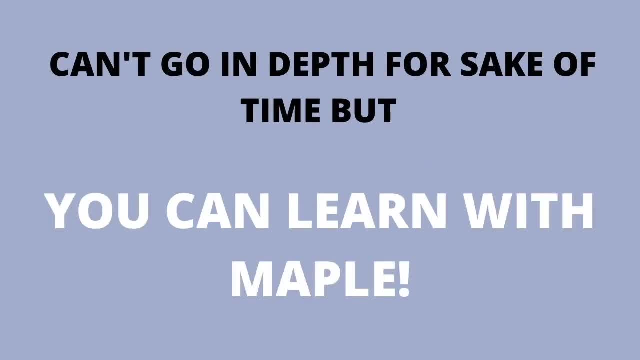 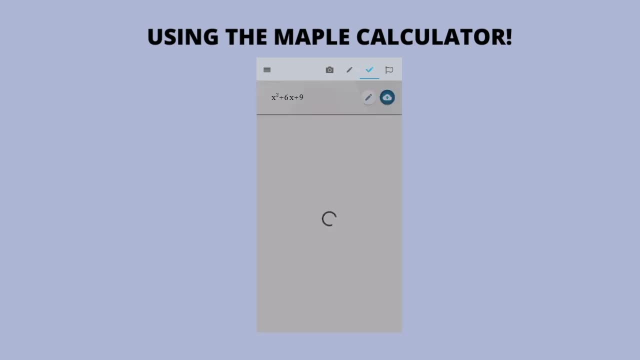 Another popular method is factoring And due to the sake of time I can't explain all the steps, but the Maple Calculator does a pretty good job of explaining it once you put an equation in. and you can check our video about factoring, which I'll link right here.